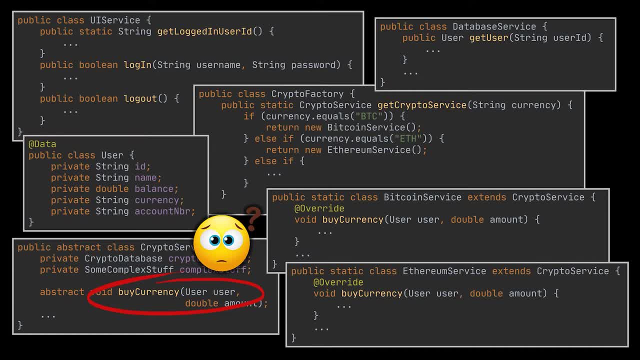 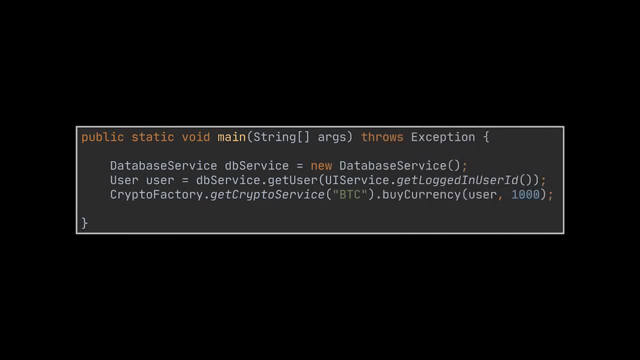 reuse the buy currency method offered by this library. how hard can that be, right? well, you can go ahead and directly call the method provided by this library, after fetching the required parameters of the services method, of course, and be done with it. however, there is a catch. what if this code was needed by other parts of our application? we can't let these parts depend. 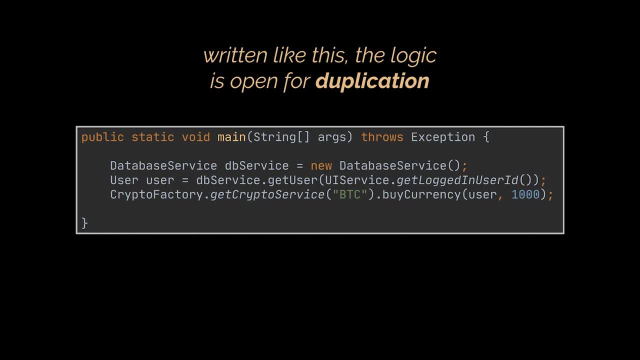 on the code we just wrote. we will have to duplicate this code here and there. right, and what about requirements change? what if we now need to check if this user has enough balance in his account to actually perform this transaction? or perhaps we now need to use the mail service? 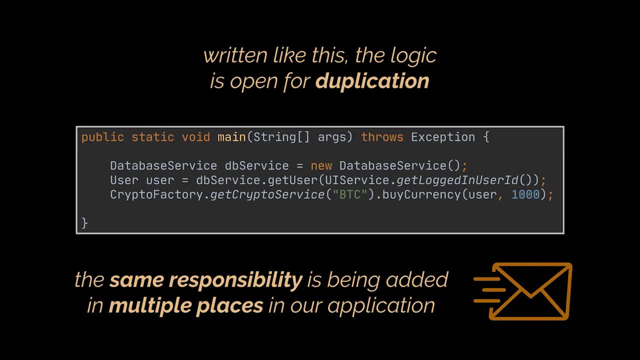 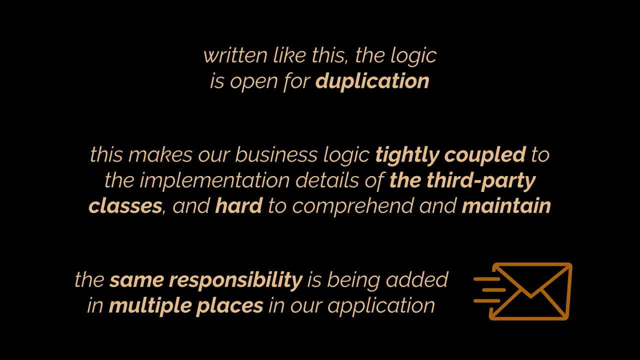 provided by the library or other parts of the library, to send an email to the customer after said transaction was made. well, we will have to change this in every part of the code that made use of this logic, making our business logic tightly coupled to the implementation details of the third-party classes. 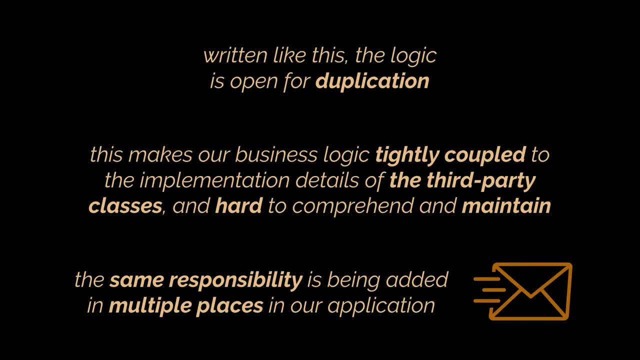 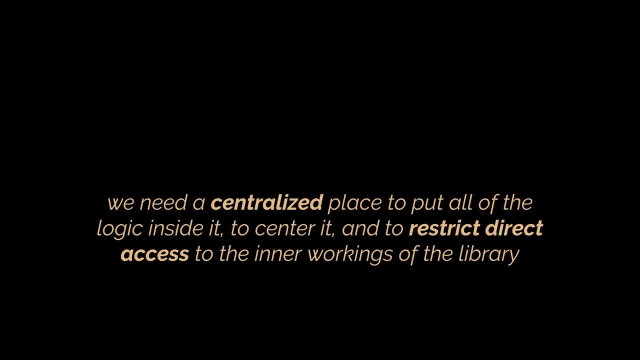 and hard to comprehend and maintain. think about it. why should several parts of our application bother working with the same logic or even have access to the third-party library we choose to rely on? so what we need is kind of a centralized place to put all the logic we require inside, not only to center it in case it was used by several parts of our app, but 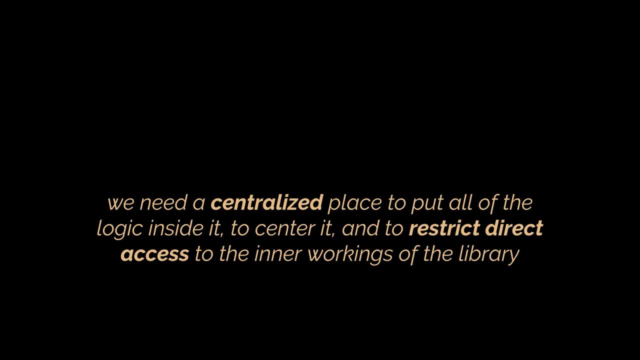 also to restrict direct access to the inner workings of the library we are working with. the centralized place, the place the clients will have access to and work with, is none other than a facade for the inner workings of our logic. it is a simplified interface for all the nasty stuff. 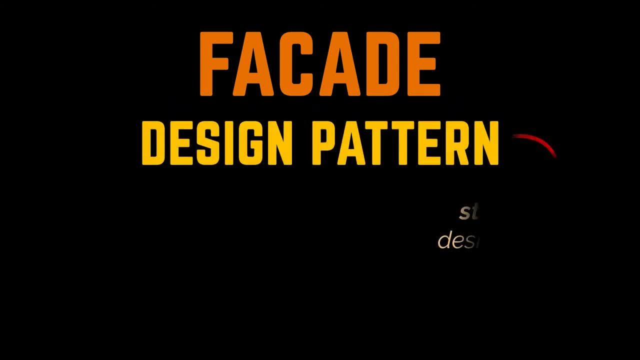 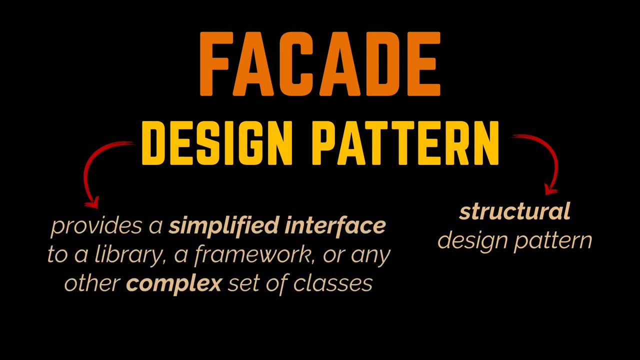 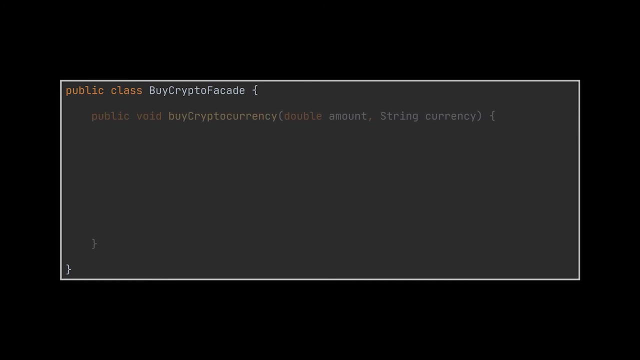 happening in the background, and that is exactly what the facade pattern is all about. this pattern is a structural design pattern that provides a simplified interface to a library, a framework or any other complex set of classes. so, in this example, to apply the facade pattern, all we need to do is create a new class. let's name it by crypto facade. in this class, we are 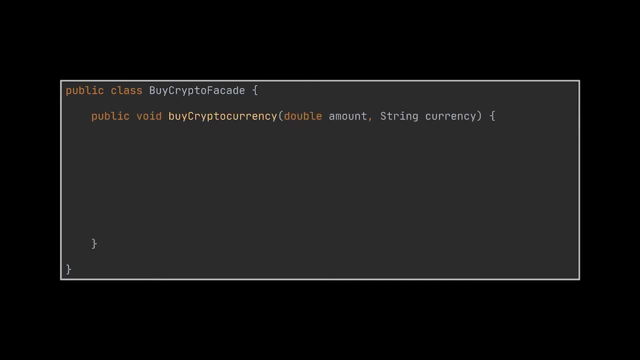 going to create a method that takes as parameters the optimal needed information to proceed with the transaction. make it as simple as possible. first we are going to retrieve the logged in user from the database, then check if the balance associated with this user allows them to perform the transaction they requested. then, if all is good, 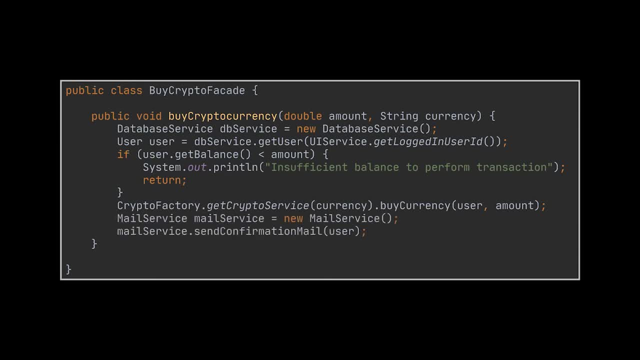 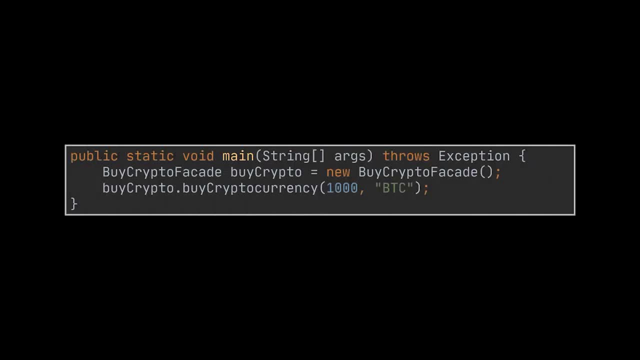 we perform the transaction and finally send an email to confirm it. now, as you can see, the client code does not have to go through all of the previous steps anymore. they just provide us with the amount they want to invest and which cryptocurrency they wanted invested in, and boom. 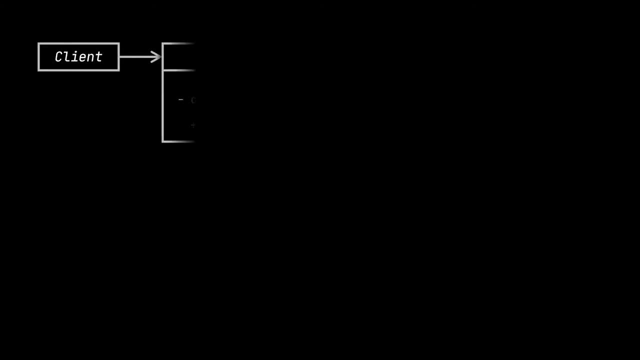 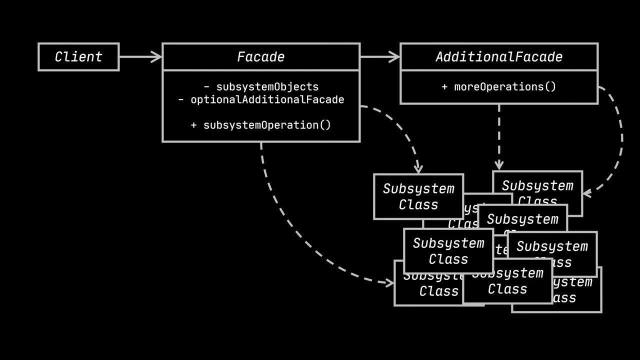 we have them covered. okay, let's go ahead and take a look at the structure or the class diagram of the facade design pattern, while trying to relate it to the example we just implemented. the first thing you will notice is the facade itself. it was represented by the by crypto. 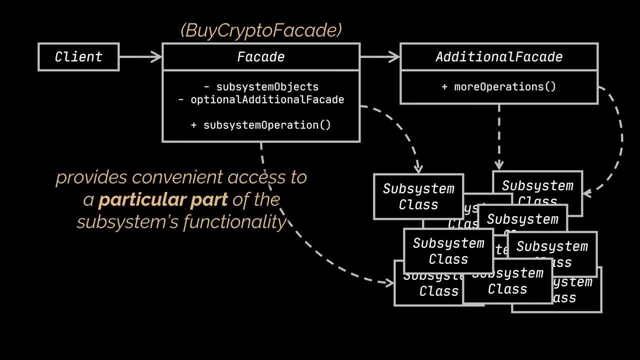 facade class. in our example, this class provides convenient access to a particular part of the subsystem's functionality. it knows where to direct the client's request and how to operate all the moving parts of this request. sometimes the facade can grow too big and become a god object, making all of our code depend on it. to avoid that, an additional facade class can be. 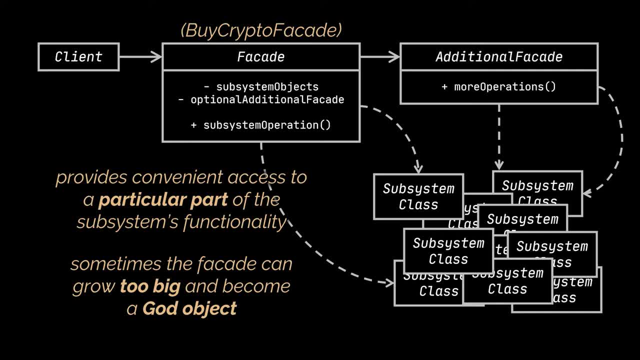 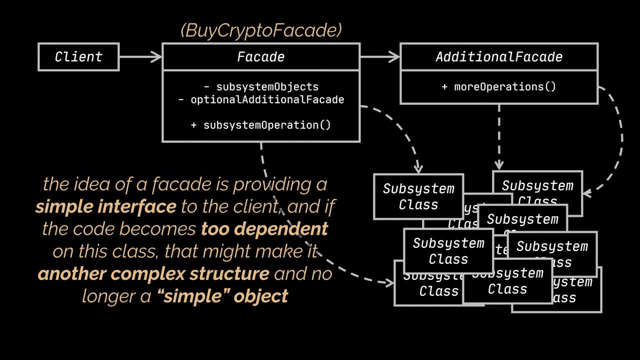 created to prevent polluting a single facade with unrelated features. remember, the idea of a facade is providing a simplified interface to the client and if the code becomes too dependent on this class, that might make it yet another complex structure and no longer a simple object. the additional facades can be used by both clients and other facades and may come in handy for such use. 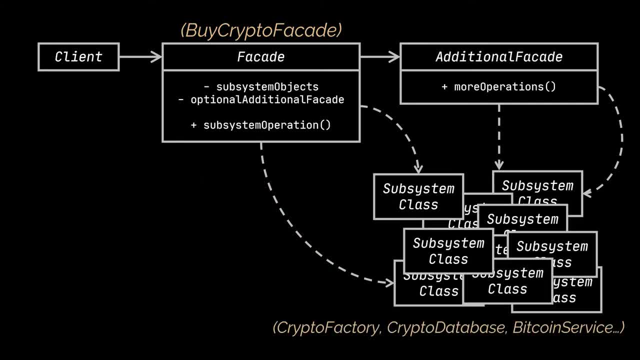 next on the diagram, you can see the complex subsystem classes. these classes were represented by the various objects and classes provided by the third party library. in our previous example. the facade initializes these objects in the correct order and supplies them with data and the proper format. subsystem classes aren't aware of the facade's existence. they operate within the 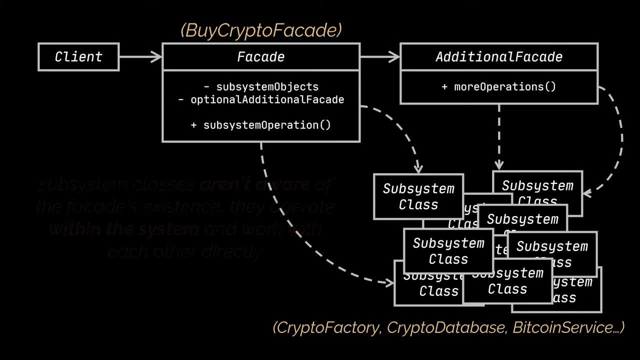 system and work with each other directly. and finally, the last piece of the diagram is none other than the client. the client uses the facade instead of calling the subsystem objects directly. so, instead of working with dozens of the framework's complex classes directly, the client creates a facade class and uses the simple functionality they need. so, to sum everything up,